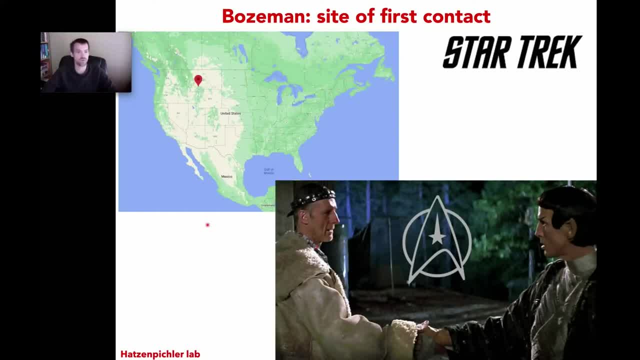 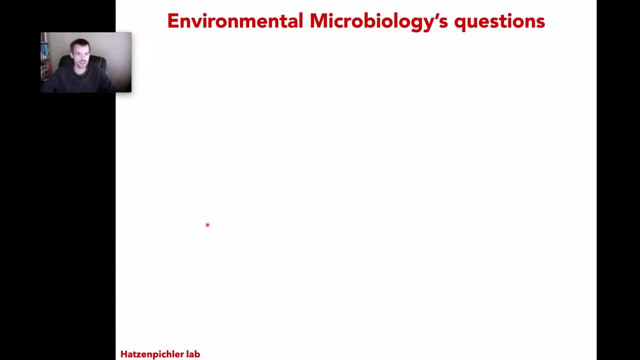 I want to talk to you about today microorganisms in the extreme features of Yellowstone National Park. Before we go to Yellowstone National Park together, I first want to give you a quick introduction of what environmental microbiologists like myself are doing. So the questions an environmental microbiologist has whenever we see a new microorganism. 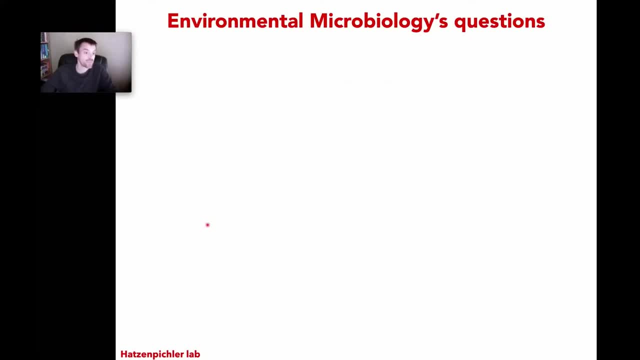 the same questions that you would ask a person when you meet them for the first time. Who are you? What are you doing? When are you doing that? Where are you located and where do you do your job? With whom do you typically hang out with? Who are your friends? Who are your? 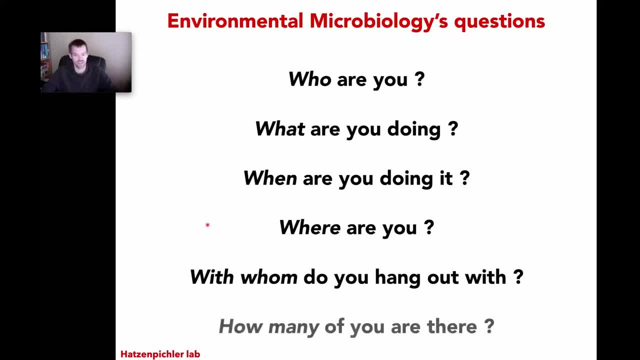 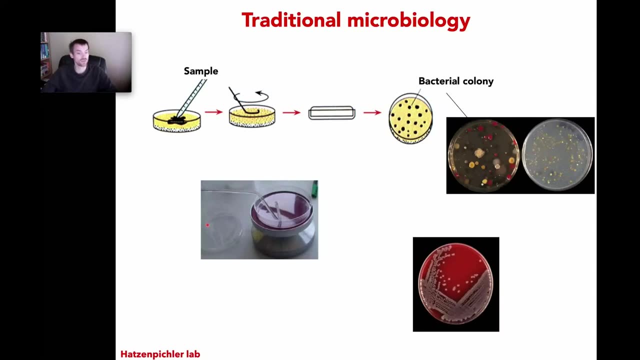 enemies, Who are your frenemies And how many of you are there in the environmental sample in the environment? and so traditionally how environmental microbiologists have approached these kind of questions was to using cultivation approaches. so we went into the environment of interest, we took a sample. that could be, you know, a soil sample or a water sample, and you know we. 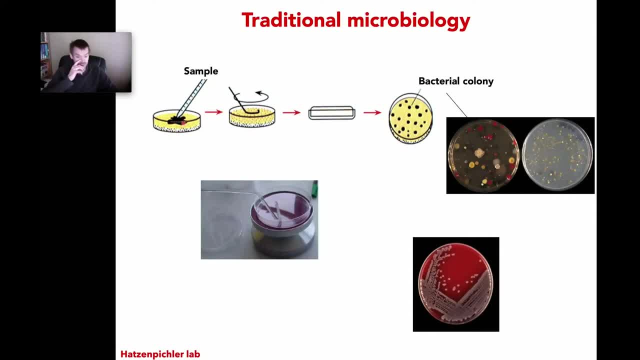 tried to grow microorganisms from that sample on a petri dish or in an elm myoflask in the lab. so we provided some artificial growth medium in a petri dish, you know. we provided them with energy sources, with carbon sources and so on. we, you know, made life as cozy as possible for these organisms. 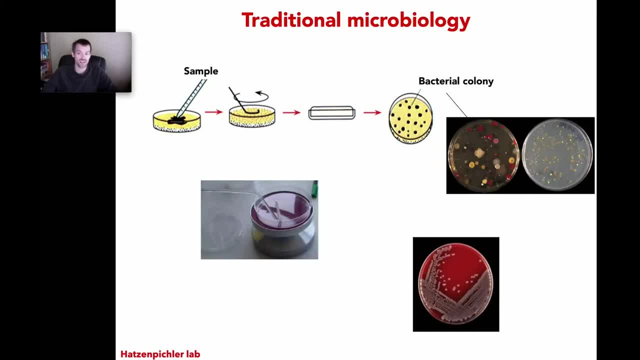 in the lab, and then you know, just waited a few days. and then you know, waited up which microorganisms might be growing up in these. you know colonies of bacteria that were growing up on the arga plate and then try to identify who they are, and then you know what are they doing, and so on. 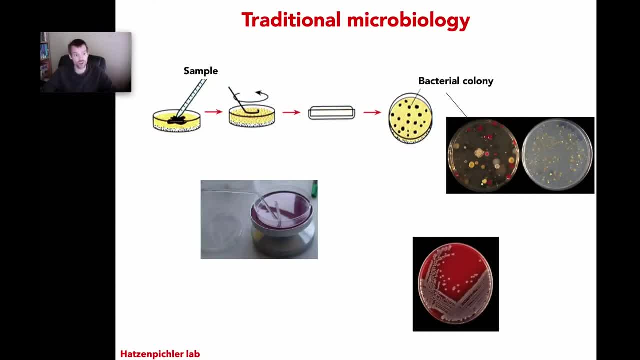 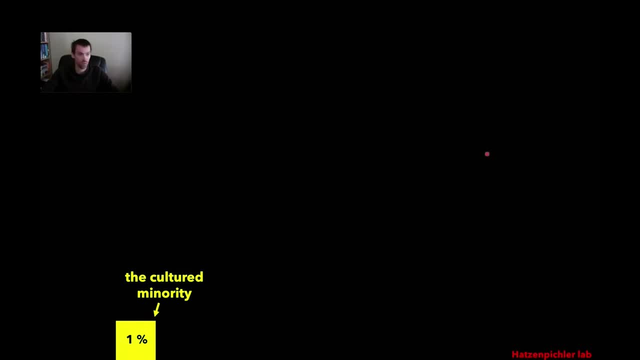 there's a problem, however, and that is that the majority of organisms that we know out there cannot be grown in the lab. so if i would plot you know all the microorganisms you know that we know exist out there and only show the fraction of the ones that we can actually grow in the lab on the artificial conditions, we would see that 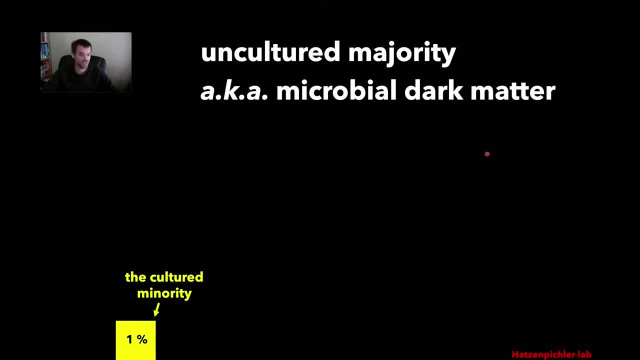 about only one percent, on average, of any microorganisms we know out there can be grown in the lab, but the majority of them is what is called the microbial dark matter, in a term that we, you know, borrowed from astrophysics, or the uncultured majority that makes up, you know, the majority of. 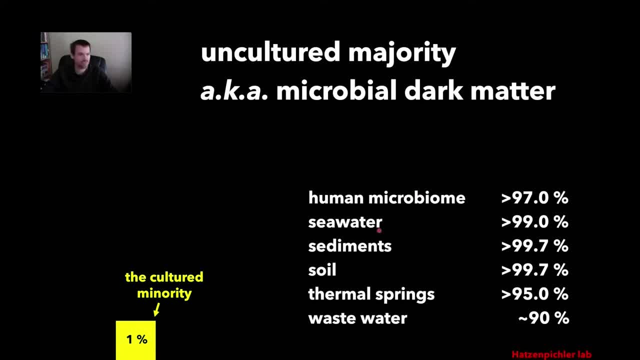 microorganisms in the lab, and that's what we call the microbial dark matter, which is particular yours. look at this one, this is this one, the one that was from a lab, one. it's called the offshares. this is the pumping plant, so it's a part of the scorpion. it's should be, אבל 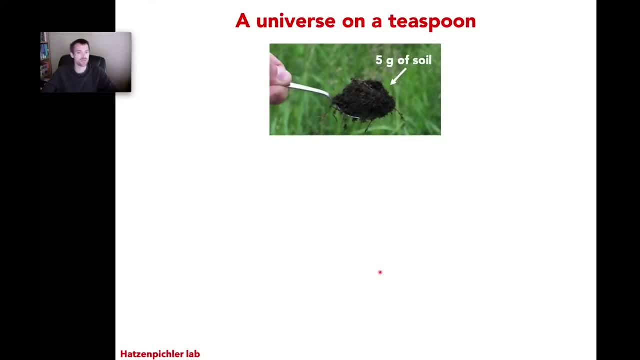 mografi responsible. but can it grow in the lab? not at all. we have like the feminist. so if we take someLED粽, for example, when you take some e in the lab, you can take just about 1.80ジم jhyun per second over the surface of this container and yeah. and if it's full carbon that we always give it some ico gene. you took that plus, you know, and you try to see if the ngàyirao and lapis- one or other terms- are at a very high profile of them leaving a pop, you know. however, do they depend on people like that to make sure you keep angry? 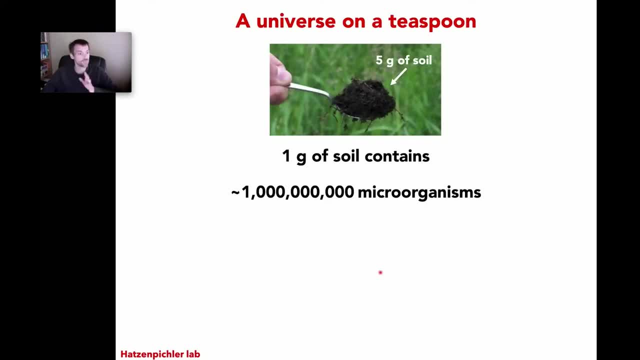 and vegetable organic microorganisms go, take care of through the the site, a lot of Chainłuja in or are members of the eukaryotes. To put this number into perspective, our galaxy has about 100 billion stars And the soil- this one gram of soil that we just scooped up- has about 10,000 to. 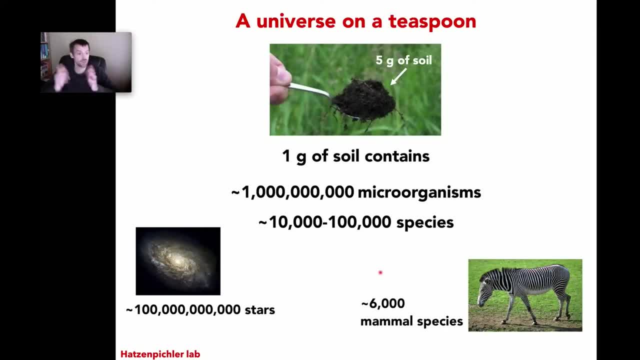 100,000 different species of microorganisms. To put this into perspective, on the entire planet Earth we have about 6,000 different mammal species. So we're talking about gigantic numbers here, And you know the Earth is obviously not only composed of soil. there's many different. 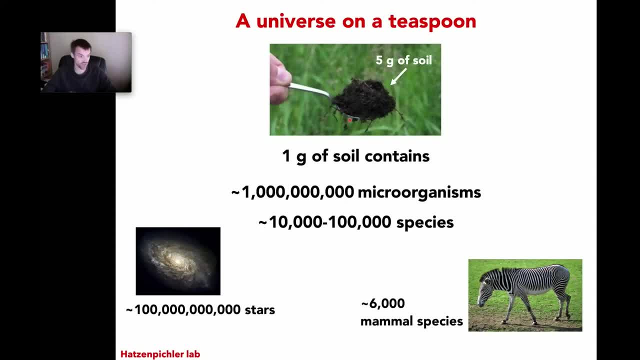 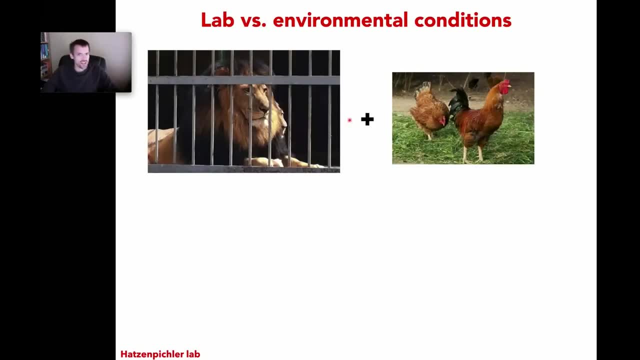 habitat types, in every one of which, as we just showed before, the majority of microorganisms cannot be grown in the lab. I first want to talk a little bit about why that is. Why is it so hard for us microbial ecologists and environmental microbiologists to replicate the conditions in 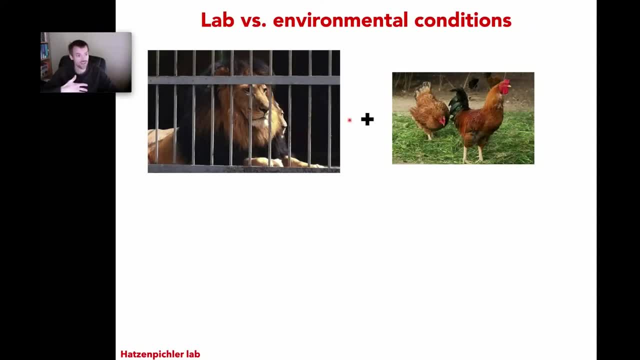 the lab And why some of the lessons we can learn by studying microorganisms directly in the lab are, you know, ultimately limited. And I want to give you this example of a lion. What for What food is a lion eating? What you know? how is it? how is a lion interacting with its 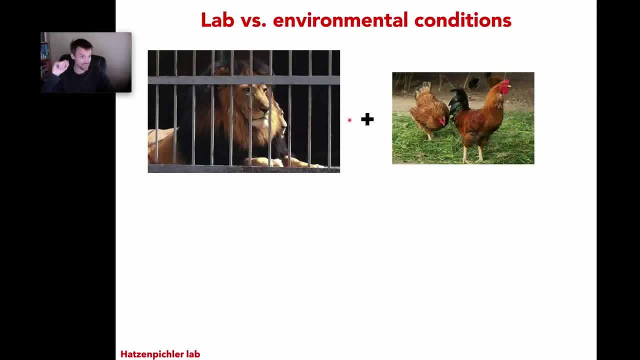 environment. What you will do is you will go into the Serengeti and you will observe a lion. What are they doing? What you will not do is you will not try to capture a lion in the wild, bring it back into a zoo, put it into captivity and then feed it a chicken, Because that condition 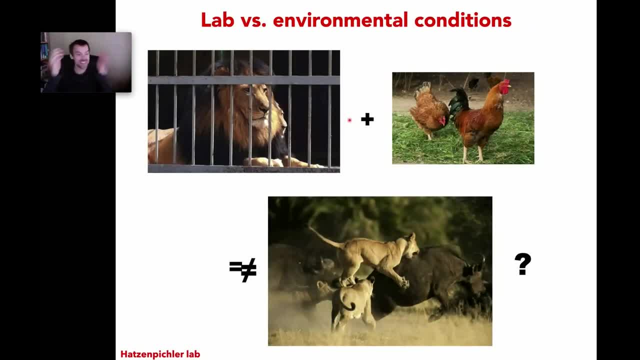 is obviously not how a lion is living in the wild, But this is exactly what we are doing if we try to go to an environment and try to isolate an organism from its environment and grow it in the lab under artificial conditions. What you learn is still important. You still learn something about. 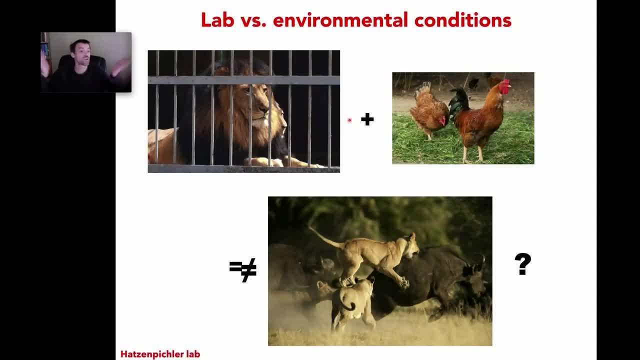 the biology of the organism right. In this case, you learn that a lion eats a chicken. Of course the lion will eat the chicken. Does that mean that the chicken is the natural prey for the lion? No, of course it's not right, And so it is very, very important to keep that in mind for microbiology. 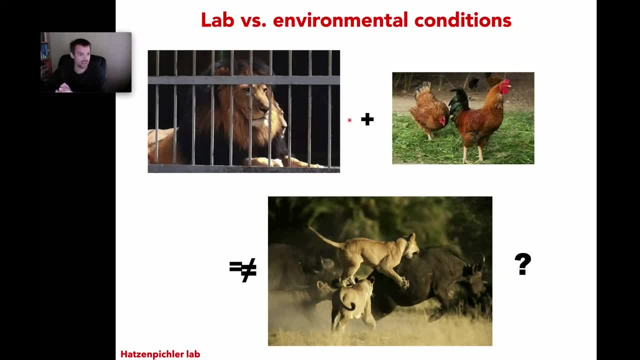 What you'll read in a textbook about microbiology. right has been done by studying organisms in captivity in a glass beaker that is shaking at 200 rounds per minute in a lab somewhere. This is not how the organism is growing in its natural 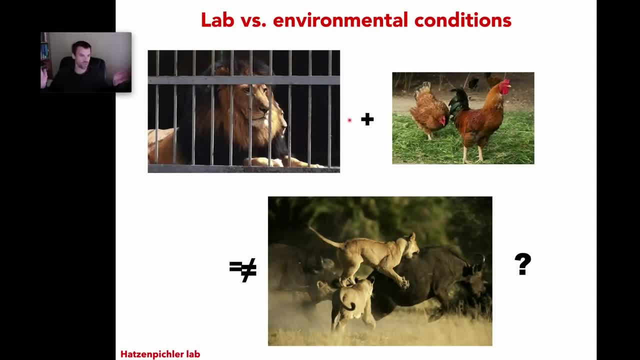 environment, And this is what we, as environmental microbiologists, want to do. We want to understand what is the organism doing in the real world, in the real conditions where it's hanging out with thousands and thousands of other species. The other problem is that organisms, microorganisms- 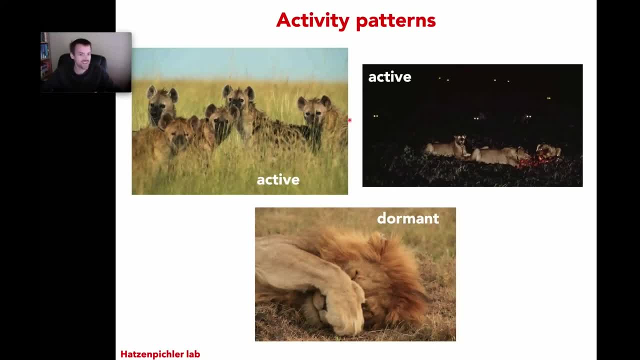 just as animals have activity patterns: Some of them are dormant during the day, Some of them are active during the day, Some of them are active in the night And some of them, you know, can be dormant for quite a long time. There have been some microorganisms found in deep sea sediments. 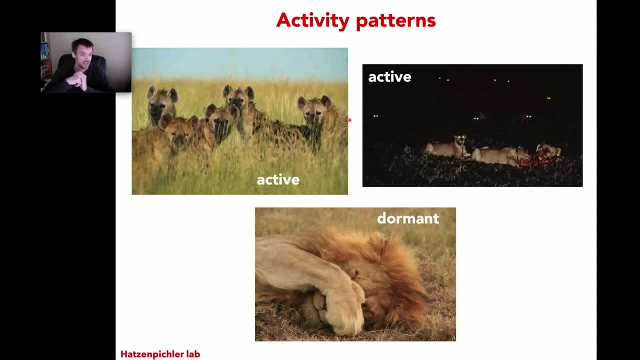 that apparently have been dormant for millions of years. But if the conditions switch to the right, the environment suddenly, you know, has a burst of nutrients that you know flowed into the environment. Suddenly the microorganisms become active because, you know, 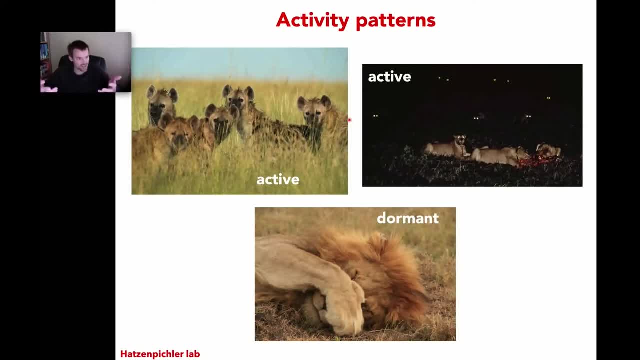 the condition changed for the better. The same concept obviously applies in zoology, right? We would never assume that all organisms are only active during a particular time of the day. Of course not. Everyone has their particular environmental niche, And the same is true for 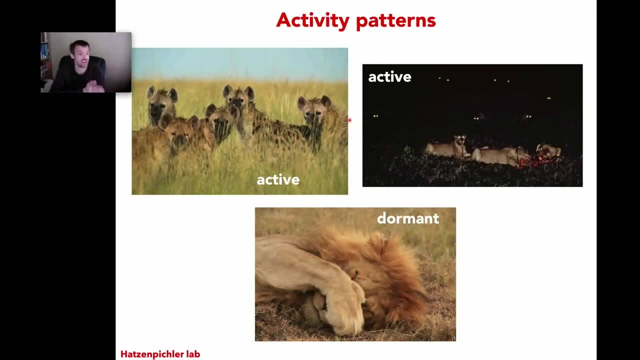 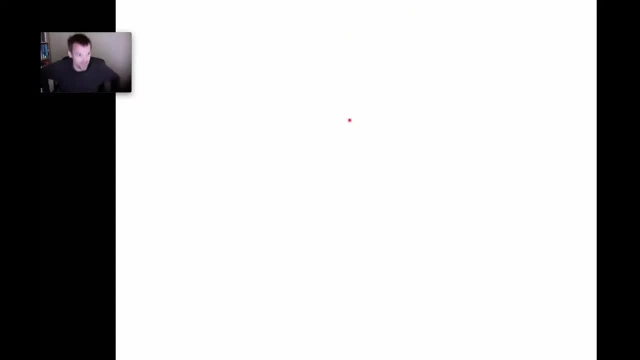 microorganisms By growing them in isolation in a beaker. you ignore all of that. You take this out of its natural conditions. What are we studying, or which kind of microorganisms are we studying, in Yellowstone National Park? Why do we study microorganisms in Yellowstone National Park? 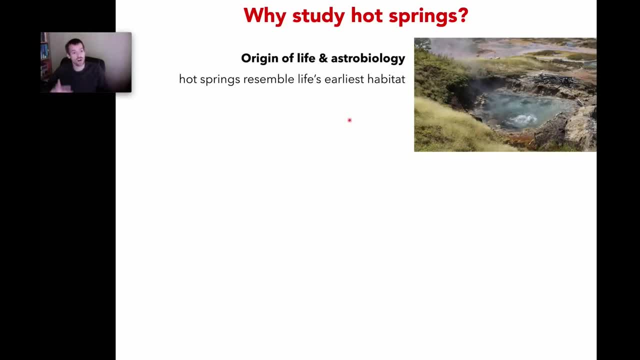 Why do we study hot springs to begin with? The first one is we know that hot springs resemble life's earliest habitat, At the, you know, at the start, after the formation of the earth, after the earth cooled down to allow liquid water on its surface, earth was pretty hot still. 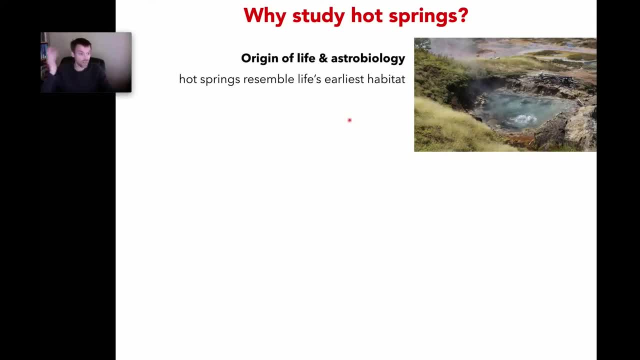 right, We are talking about, you know, 80,, 90,, 100 boiling temperatures of water temperature, And this is the habitat where the early life forms, the first microorganisms formed. So by studying extant life in hot springs, we learn something about the origin of life, the origin of 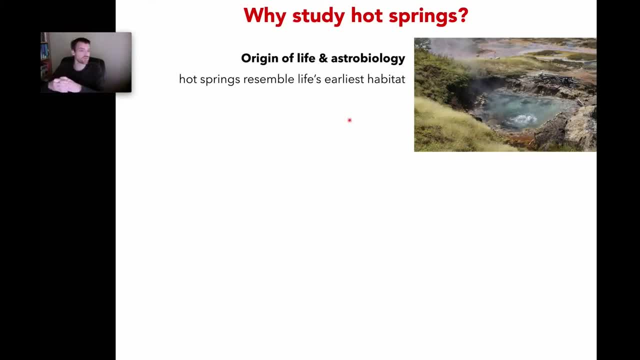 cells in the ancient habitat where earth evolved 3.5 to 4 billion years ago, And we learn what the implications of that are for astrobiology, So for the study of life in the universe. Are there any other planets, any other celestial bodies out there that could also be home to? 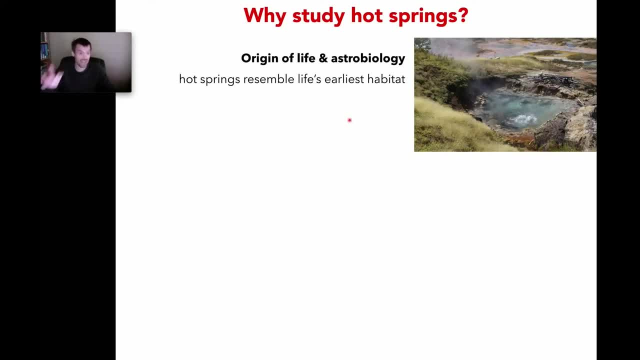 alien life forms, And by studying the extremes of life on the planet earth, we can learn what are the extremes that we can expect on other planets, Like, for example, planet Mars, or when we talk about hot environments we typically talk about 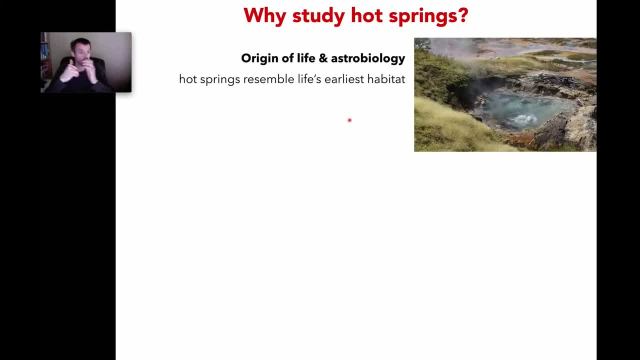 you know, the Jupiter moons like Europa, where we think there is, you know, deep sea hydrothermal vents on these moons. Another reason is that, as I just mentioned before, the majority of microorganisms on the planet cannot be grown in the lab, And 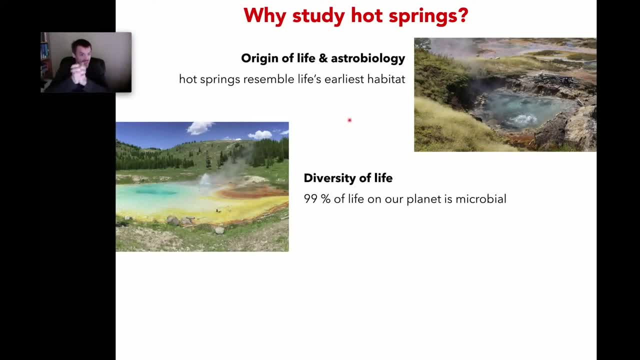 as you know, 99% of the life on the planet is microbial. So 99 percent of the 99 percent of life on the planet came from microorganisms that cannot be grown in the lab. So if we go to the environments that provide the most extreme conditions, we can explore the entire scale. 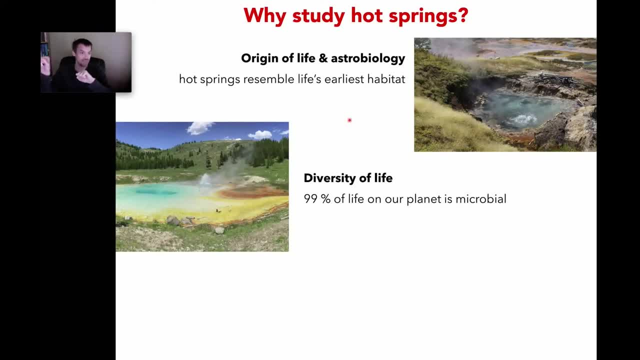 of diversity of life that exists on the planet. We want to look at the deepest habitats on the planet in the deep sea. We want to look at the coldest places, in glaciers and theatrica, in geothermal hot springs that are on the other side of the temperature spectrum. 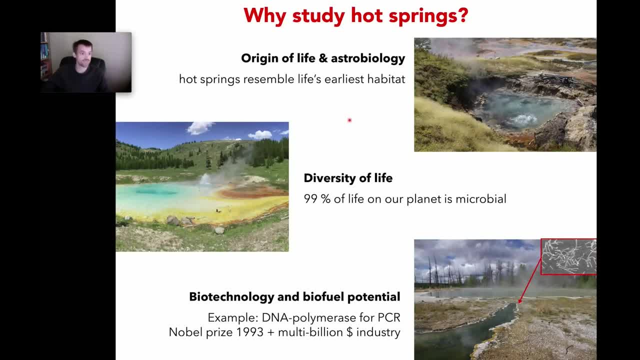 In the last one. hot springs are a great reservoir for potential biotechnology and biofuel industry. The most prominent example for this is DNA polymerase, the Taq polymerase that a scientist called Thomas Brock found in the organism Thermos aquaticus that he isolated from. 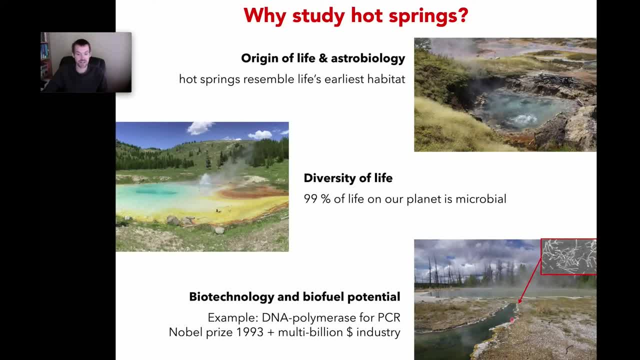 mushroom hot spring here in Yellowstone National Park and in which, a few years later, isolated the DNA polymerase from on which the PCR, the polymerase chain reaction that we today use in labs worldwide to amplify DNA, is coming from. So not only did this discovery and the development 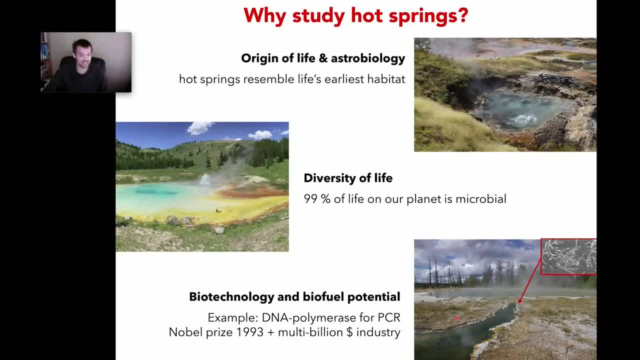 of PCR was awarded the Nobel Prize in 1993, the production of this one enzyme, this one thermostable enzyme from this 70 degrees hot spring alone, is a multi-billion dollar industry today, which shows that the potential for this discovery in organisms and their enzymes, and how they can be used for biotechnological purposes. 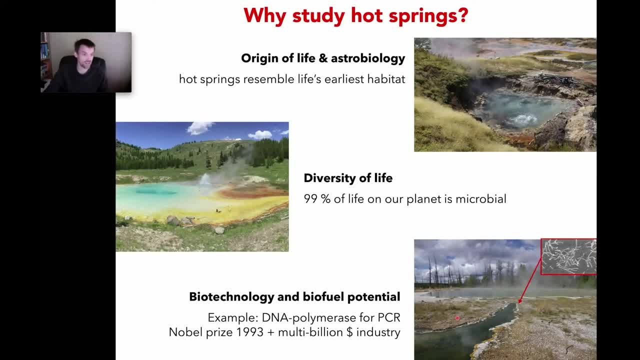 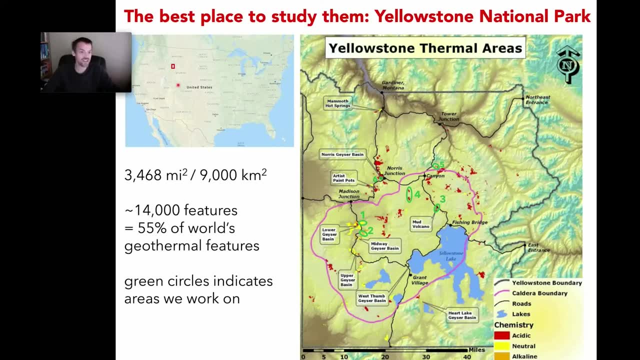 with tremendous potential for health and for the economy as well. The best place to study microorganisms that are living in hot springs is just, you know, a one hour 20 minutes drive south of Bozeman, where I live in Yellowstone National Park. that is just located at the intersection. 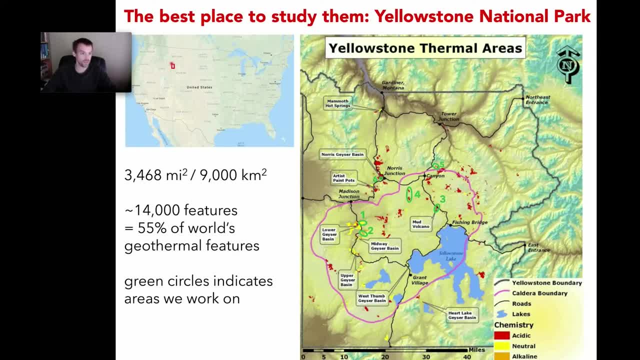 of the US states of Wyoming, Idaho and Montana. The park is about 3,500 square miles, or about 9,000 square kilometers large. To give you an idea, this is larger than the states of Rhode Island and Delaware combined and is larger than several of the states in Germany or France, for example. So 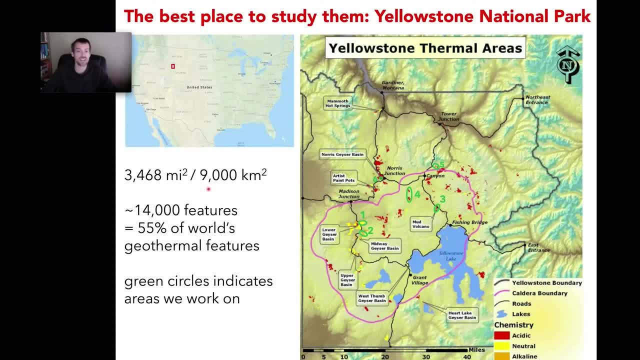 we're talking about a pretty big territory. Yellowstone National Park features about 14,000 geothermal features and is estimated to hold about 55 percent of all the world's geothermal features. And you see this map here that shows you the basic outline of Yellowstone National Park, with 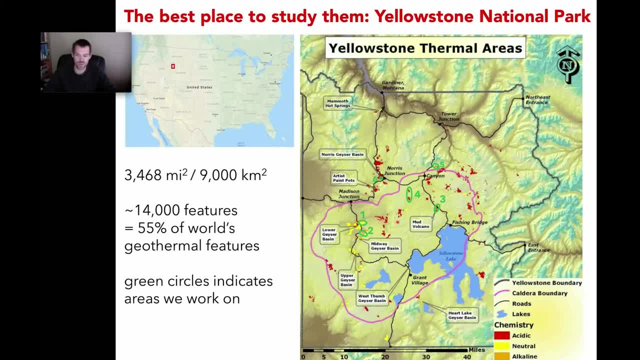 a big lake in the center, and then all these red and yellow and orange colors indicate the biggest geothermal fields in the park, So where you have clusters of hot springs and geysers, basically, And these green circles that are numbered here are the main locations where my lab is currently. 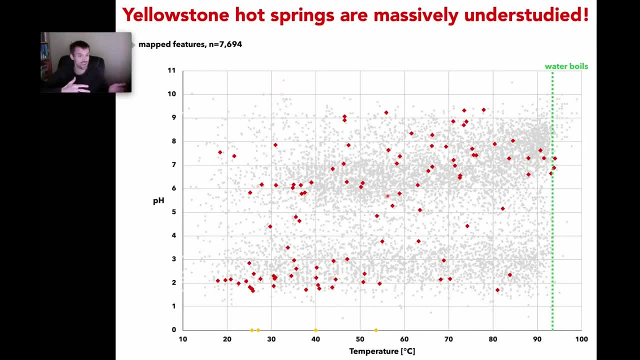 performing research, We said there's about 14,000 features, about 7,700 of them, so give or take about half of them have been logged, Meaning we know where they are and we know what their temperature and pH is. What you see in this plot is the gray dots are 7,694 plots of every geothermal feature. 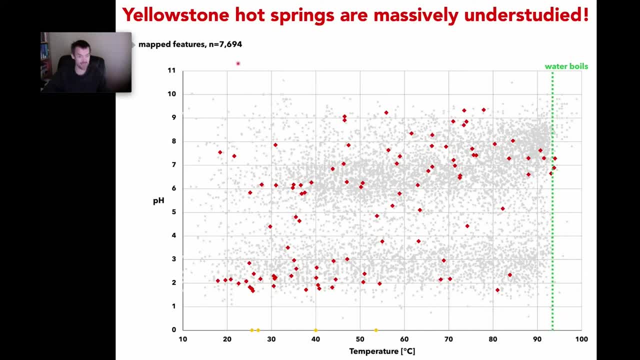 in Yellowstone National Park that has been logged, And on the x-axis you have the temperature and on the y-axis you have the pH, And so what we see there's, you know, a huge, huge diversity in terms of the temperature and the pH of the geothermal features. But one problem is that, historically, 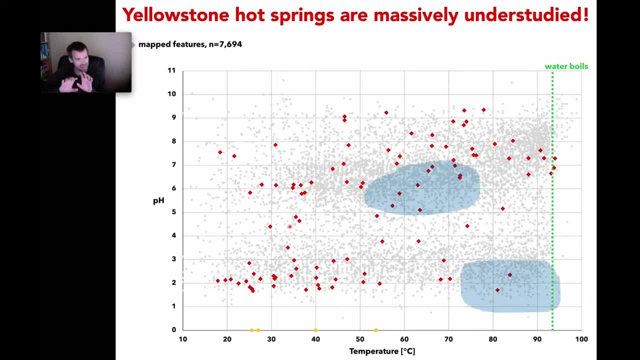 researchers have focused on a particular temperature. So we have a few particular, very particular sites of hot springs, One of them being very, very hot, so in the range of 80 to 90 degrees of boiling temperature, with a very, very low pH, So very 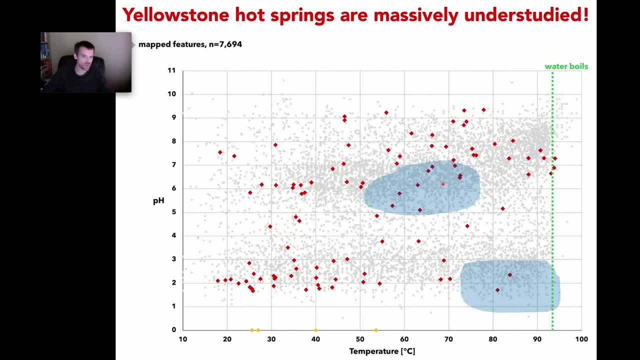 acidic features In the other ones, you know, circum-neutral, around pH 6-7-ish and a temperature of about 50 to 70 degrees Celsius. These features here have been mainly studied for the reason that they're- you know, they're- so extreme that they can only host a very low temperature. 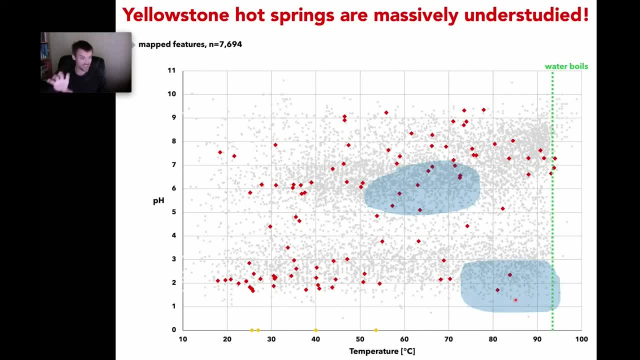 So what we see here is a huge diversity of microorganisms. In some of these features that are extremely hot and extremely acidic, you literally have like only three or four different species of microorganisms. Compare this to the soil I just talked about, where you have 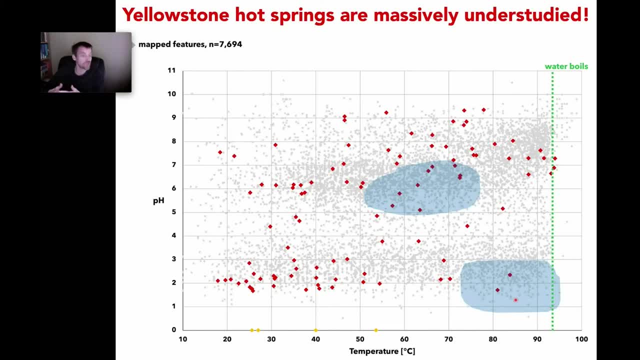 a hundred thousand species in one gram right. This is a very simple community which makes your experiments easier to conduct because you're only dealing with three or four species rather than a hundred thousand. And these features in the center here have been mainly looked at because these are 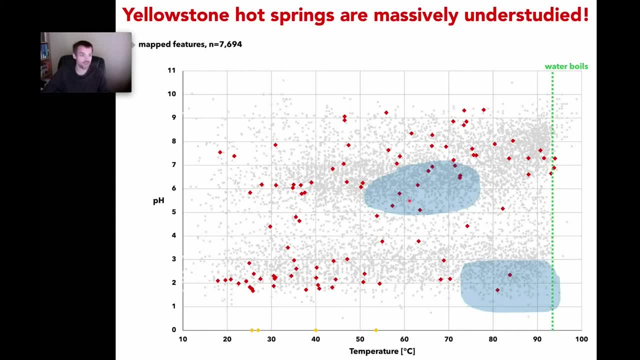 the most common features in the park. So this is a big problem I'll talk about in a minute. So after my lab was founded about three years ago, my lab has been conducting a very large survey of Yellowstone features, Yellowstone hot springs, to basically circumvent this problem. 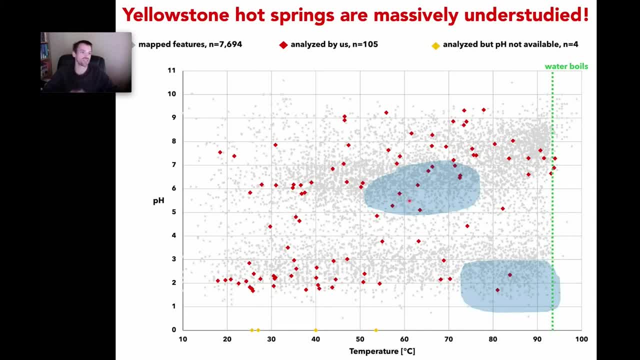 that historically, we only have looked at a very small portion of features in the park, And so all the red dots here are indicating hot springs in the park that my lab has sampled And you'll see that these are very common features in the park. So what I'm going to do is I'm going to try to get a. 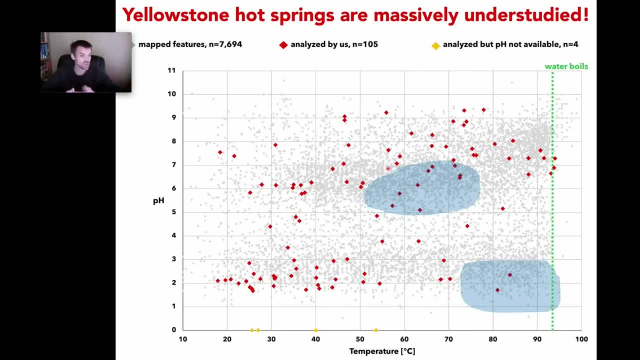 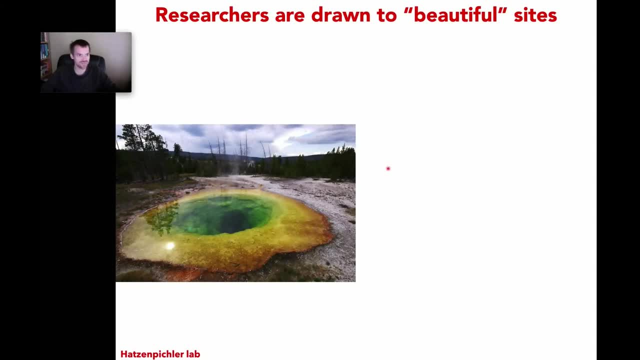 very broad representation, basically, of all the features in the park to understand the geochemistry and the microbiological inhabitants. And so one of the things we found is that researchers are also humans and we are just drawn to beautiful, quote-unquote, aesthetically pleasing sites, So many of the sites in this area that I pointed out before that are you know about circle? 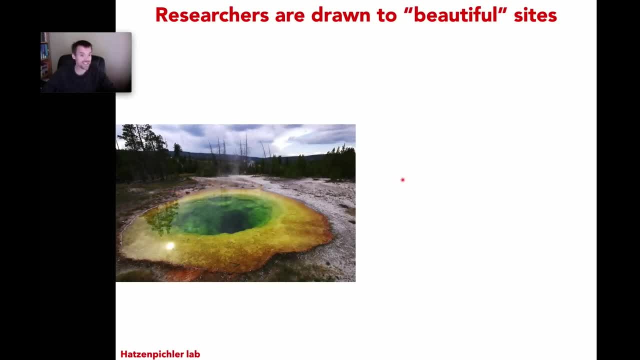 neutral 50, 60, 70 degrees Celsius, and the reason for that is that at 70 degrees, just at the end of where this blue plot is here that I just showed you, pigments break down. So most of the colors that we typically see in many 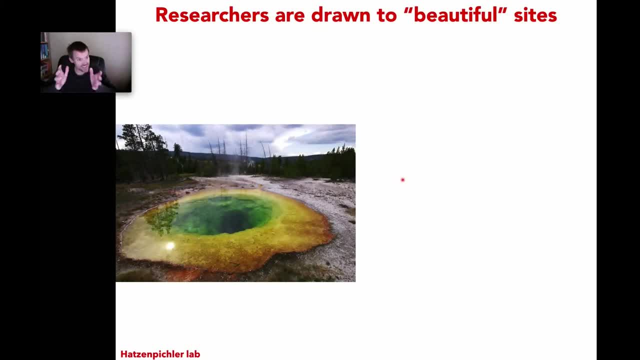 of those hot springs disappear, And so you're in this niche where you have brilliant, vibrant colors just before the pigments break down, which, you know, makes these hot springs beautiful to look at, And so, historically, a lot of researchers have focused on these gorgeous sites simply because they're nice to look at. 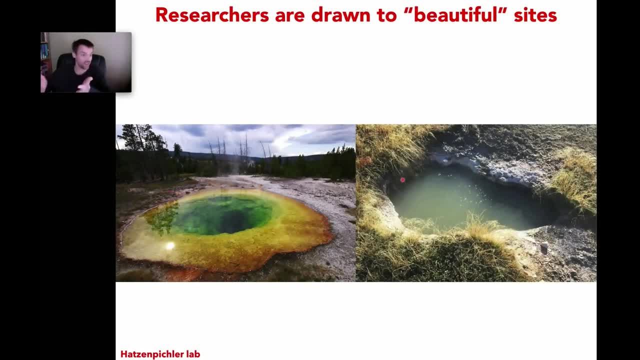 The problem is just a few meters away. there might be a hole in the ground, like shown here. that is basically a pit that is a meter in size that is filled with muddy water that also has about 60, 70 degrees Celsius. You see some gas bubbles forming here, and if 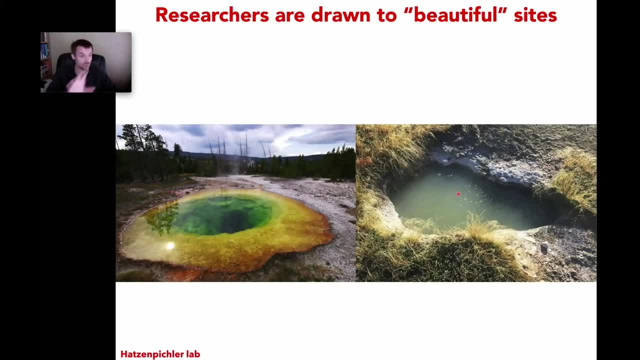 you actually look into the microorganisms that live in one and the other hot spring, you learn that the ones in the left, in these gorgeous vibrant colors, are already known to science for a long time, Because researchers have been studying this for centuries, and it's pretty crazy to see that. 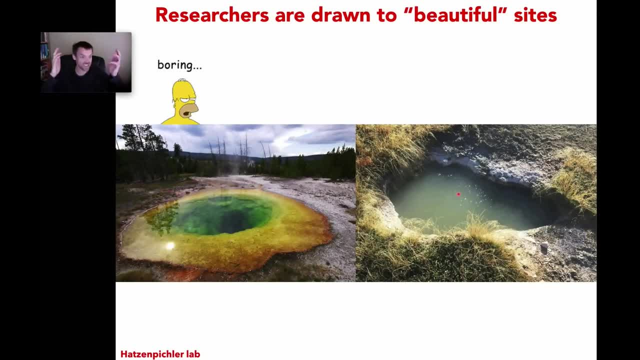 Because researchers have been studying this, for you know, 50,, 60,, 70 years, since the 1960s when modern microbiology in Yellowstone National Park started. So from you know my very high standard as an environmental microbiologist right. the organisms in the left are pretty boring. 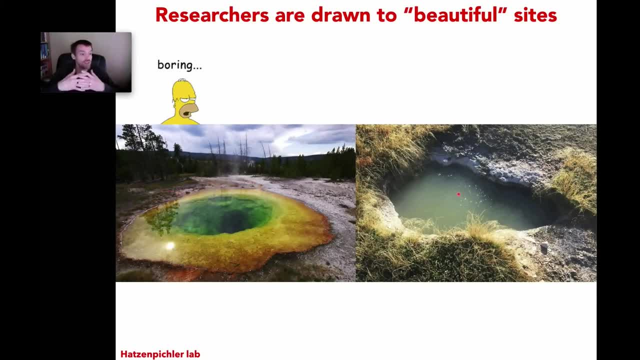 They are still pretty awesome, don't get me wrong. right, But in terms of their novelty they are not really that interesting. We know them for a long time In turn. when we look at that hole in the ground, that is just dirty mud water at 70 degrees Celsius. we actually found so much new microorganisms in this small little pool here that the diversity of new phyla, of new lineages of microorganisms in this pond, is larger than the entirety diversity of mammals on our planet combined in this one little mud pond. 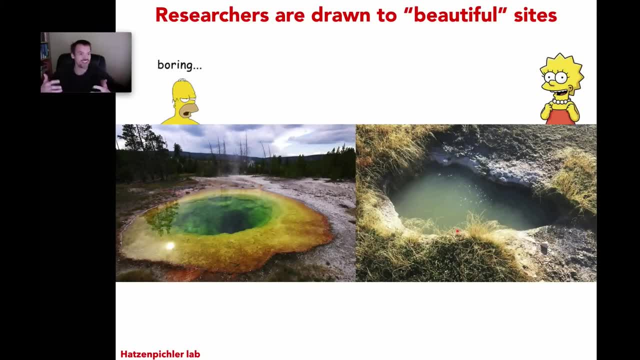 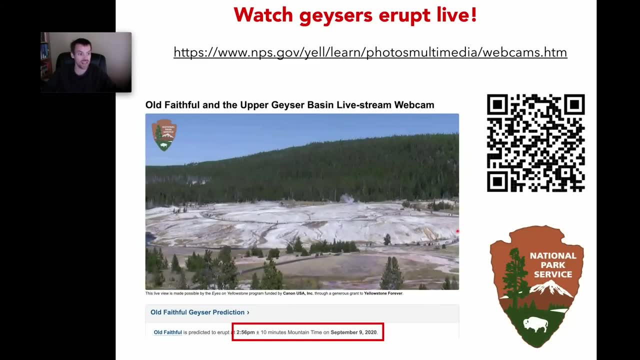 And so this shows you the tremendous potential that You know we as microbiologists- as microbiologists in particular- have when studying these diverse features. If you're interested, you can actually go online and watch Yellowstone live. The National Park Service of the United States has installed a webcam in the Geyser Valley at Old Faithful Inn, which is one of the most prominent geysers in the world. 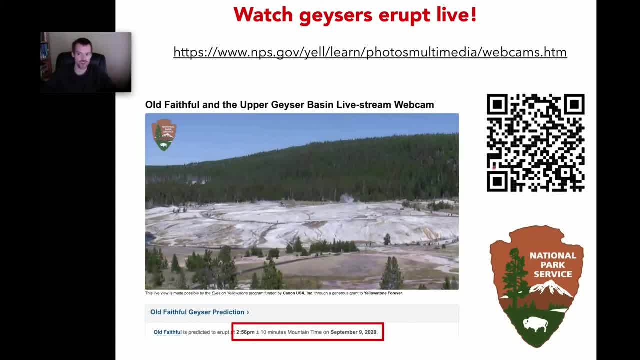 And if you go to this address, or, alternatively, you can just use your phone and scan this QR code, you can start the webcam And it will give you a live view 24 hours, 365, through the entire year. that shows you a live view and you can actually watch the geysers in the park erupting. 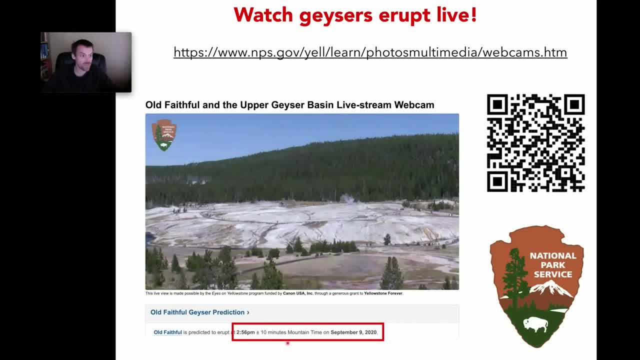 The National Park Service is nice enough to even provide you an update when the next time the eruption occurs. The next eruption of Old Faithful will happen at 2.56 pm plus minus 10 minutes. So I encourage you, if you're interested, go to this website, check when the next time Old Faithful is breaking out, be there a few minutes early and then see you know. Old Faithful is breaking out. 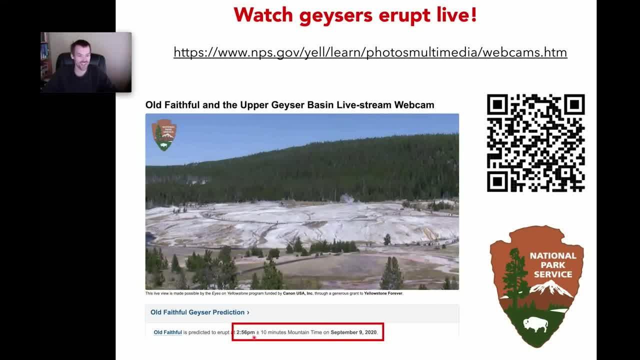 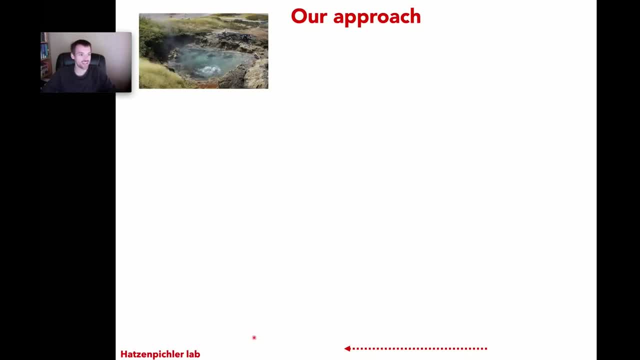 But again, it's not the first time Old Faithful has broken out in Yellowstone National Park. It's a really tremendous. it's a really tremendous sight. The last thing I want to mention is how do we study microorganisms? So one of the things we do is we go to a hot spring and we basically take DNA from this sample. we obtain biomass and sequence the DNA of the microorganisms that are contained within there. 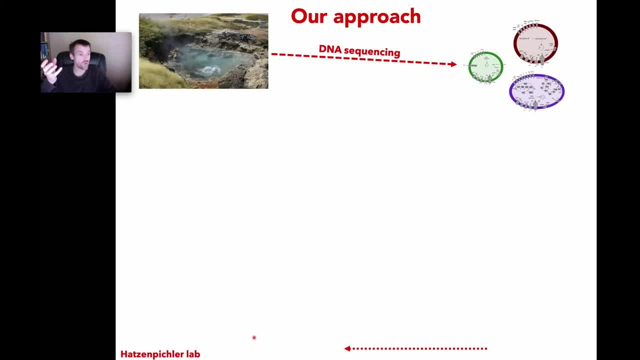 Using this DNA, we then determine what is the genomic potential, What kind of reactions can the organism run, What are potential energy sources, What are carbon sources And so on, And we then use different assays to test: are these processes actually happening in the hot spring? So, for example, 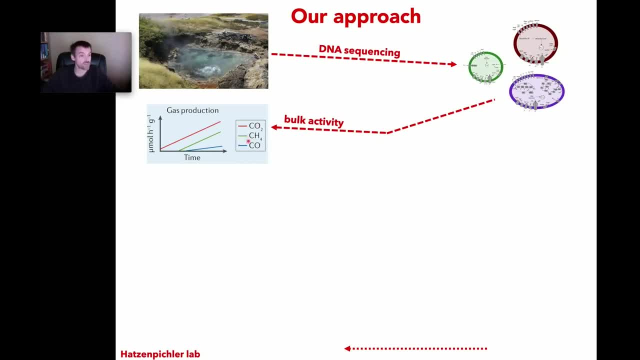 we observe whether certain gases that we predict can be produced by these microorganisms are in fact produced in this hot spring. We use sophisticated fluorescence microscopy techniques to visualize where the microorganisms are in the environment. If and how do they hang out with other cells. So this goes back to these friends and frenemies questions we had before We run.